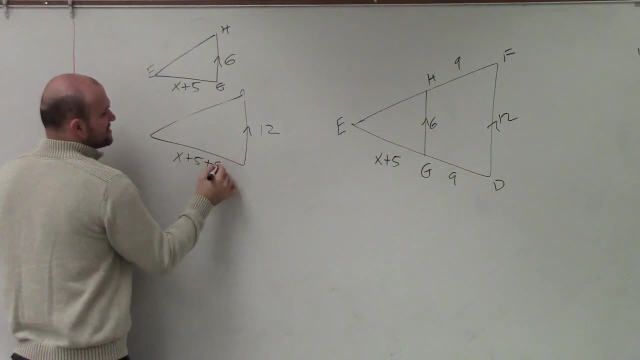 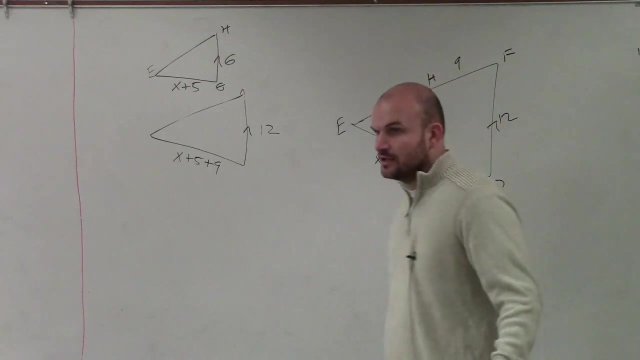 this is 12, and this is X plus 5 plus 9.. Would everybody agree with me? So, since they say that these are similar triangles, we know that they are proportional to each other. We just need to find the missing value. 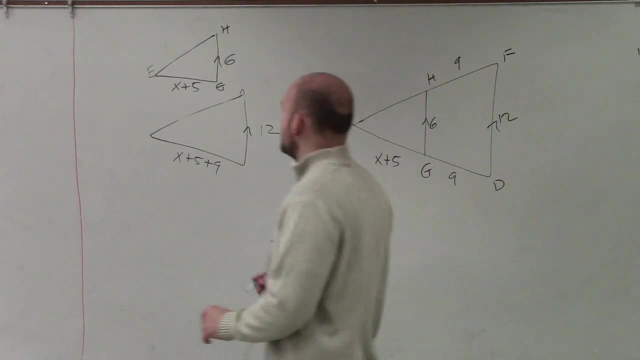 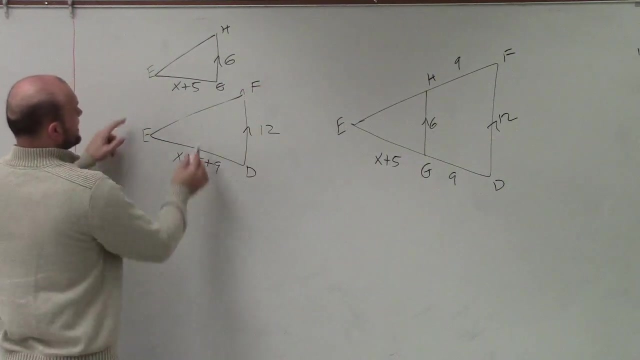 Correct. So what I can say now is: let me label this. That'd be E, D and F. So what I could say is: EG is to ED is equivalent to HG, which is to FD. right, This side is to. 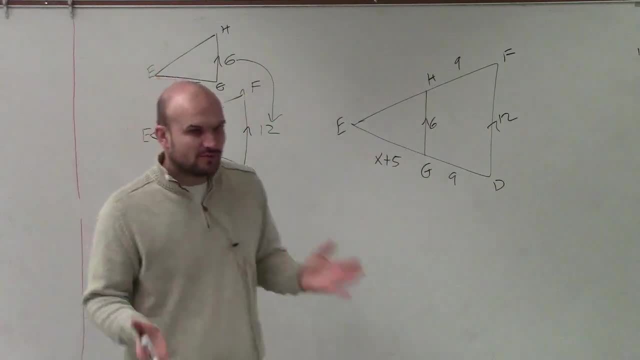 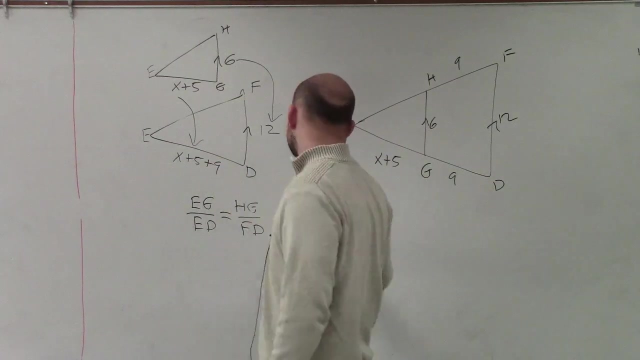 that side, as this side is to that side, Their ratios are equal, or what we call proportionate. all right, So now what I'll go ahead and do is just figure out what EG, So that's going to be. X plus 5 over this becomes X plus 14, which is equal to 6 over 12.. Now I go ahead and cross multiply. 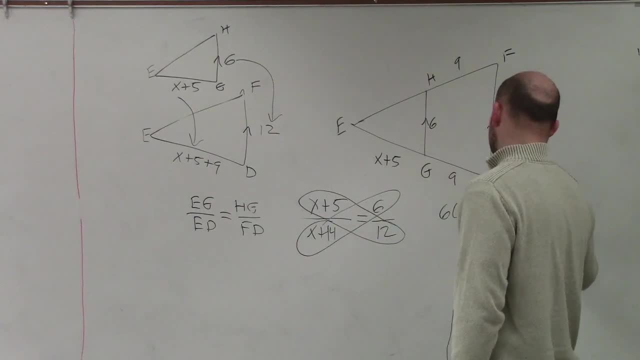 And I get 6 times X plus 14 equals to 12 times X plus 14.. And I get 6 times X plus 5. Apply distributive property. This becomes 6X. 6 times 14 is going to be 84.. 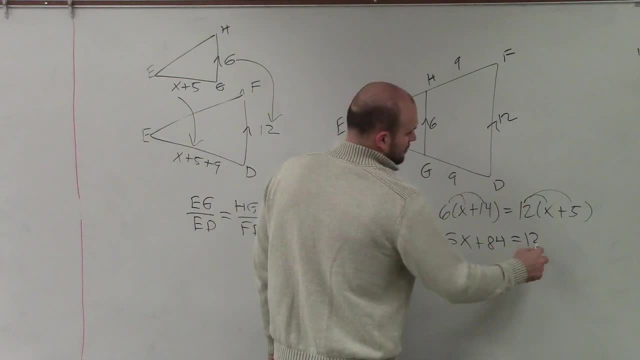 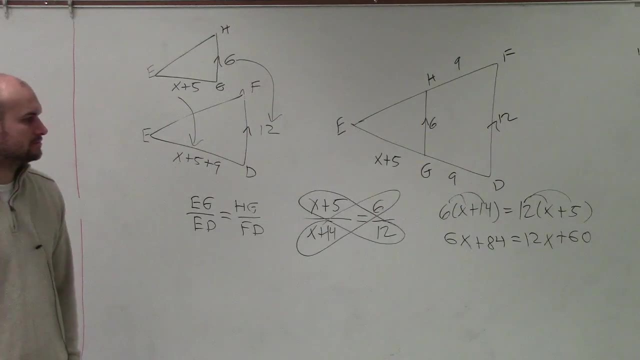 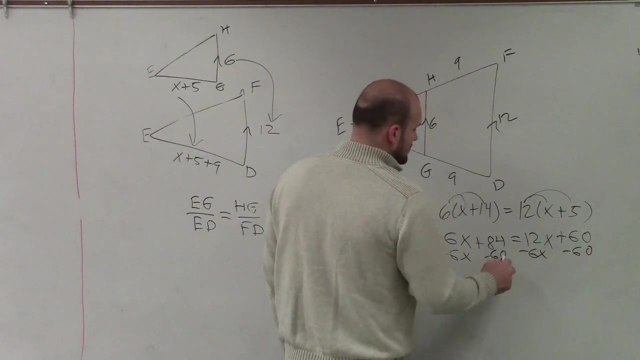 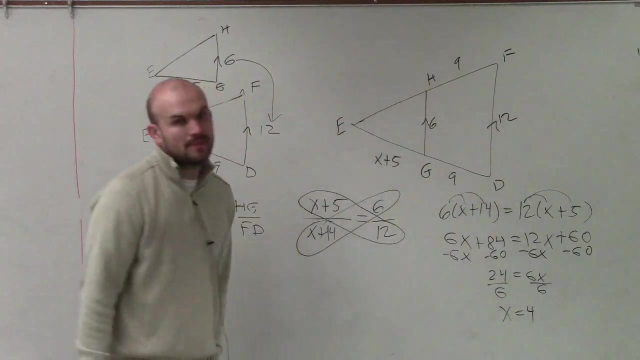 OK, So now I get this. I get the X's on the same side, so I'll subtract the 6X on both sides. I'll subtract the 60 on both sides, So I have 24 equals 6X. divide by 6,. divide by 6.. X equals 4.. Any questions? 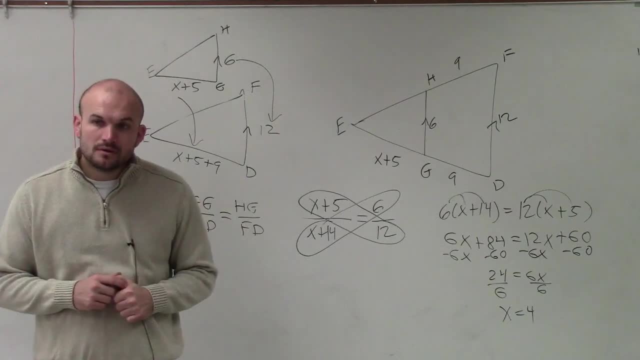 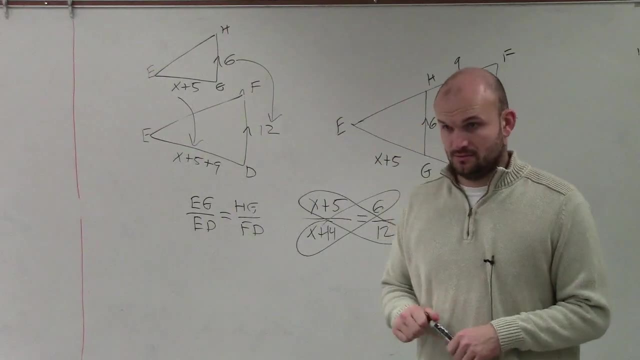 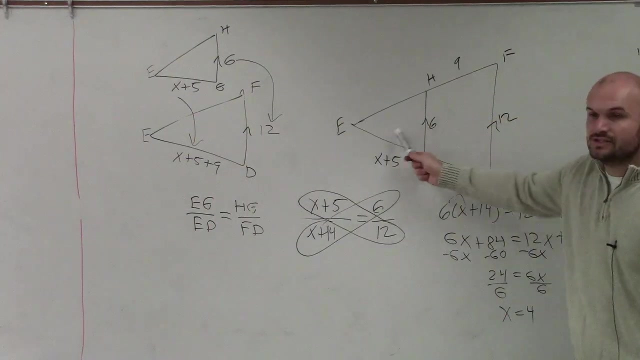 Taylor, Are they one, two or three? OK, Do you remember? similar triangles are proportional to each other. No, No, No, OK, This is question number seven. So if you look at this triangle, these two triangles, the small triangle and the large,